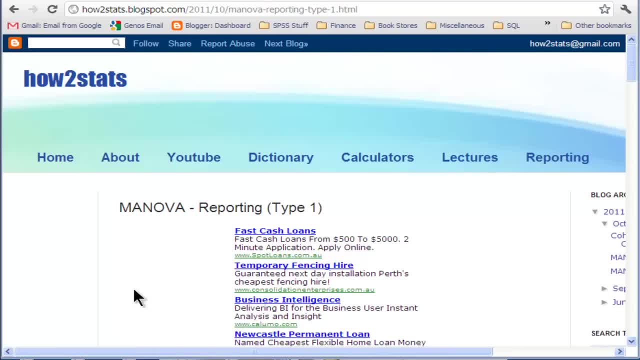 So that was videos 1,, 2,, 3, and 4 for the MANOVA on the HowToStats channel, And this is how you would write up the results for that type, what I call type 1.. I might have a better name for that, maybe GLM type 1 or something like that. 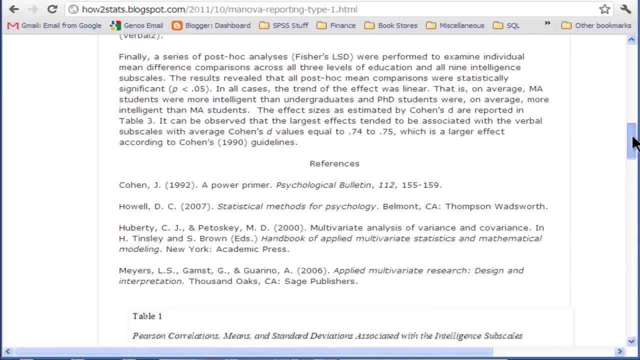 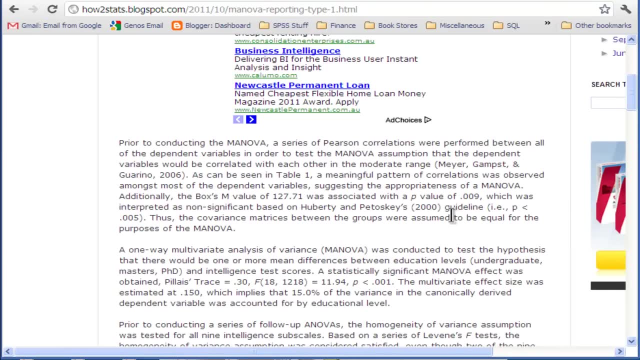 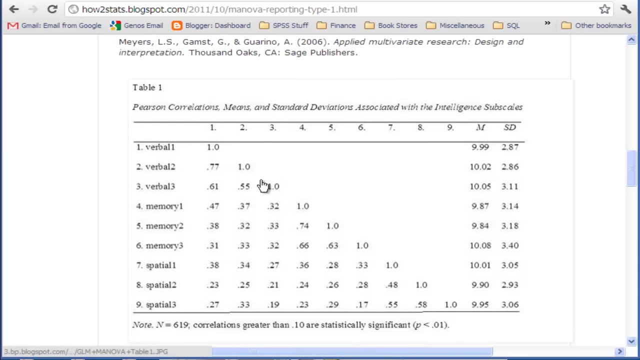 But I've written up the results for this type of analysis, with the references in the tables, and I guess the key points are. in my opinion, you should always report the correlations and the opinion of other people too. So the first thing you would do is report the correlations and the means and the standard deviations. 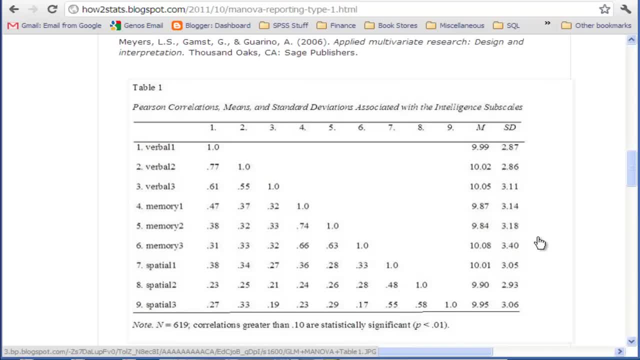 amongst your dependent variables, and you can do it like this, And this is a little trick: when you've got names for all your variables, which you almost always do- If you add numbers to them in the first column, well then you can just use numbers in the row. 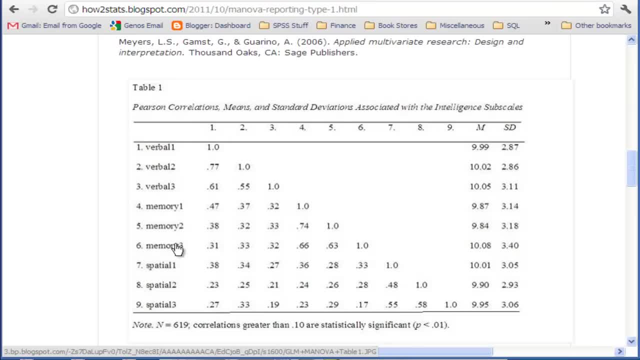 and you can save a lot of space that way. So someone could see: oh, 8 is actually spatial 2.. So it's quite easy to navigate this type of table and it's actually much smaller than it would otherwise be. And here are the means and standard deviations in the same table on the right side: 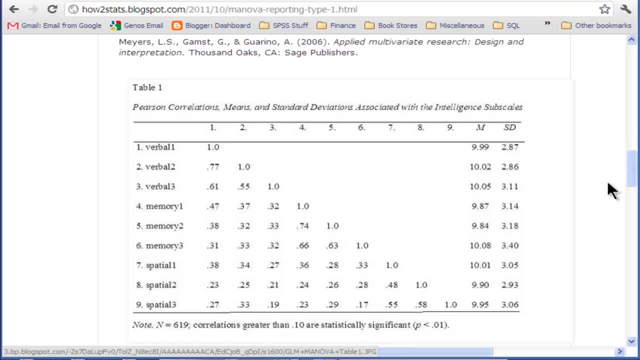 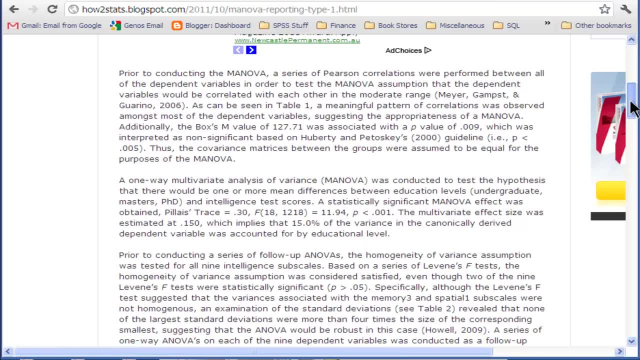 so that's clearly demarcated. You're looking at something different here, So that's a real cool way of presenting results, in my opinion, for a manuscript or a report. So after I talk about the correlations, I go through boxes M value. 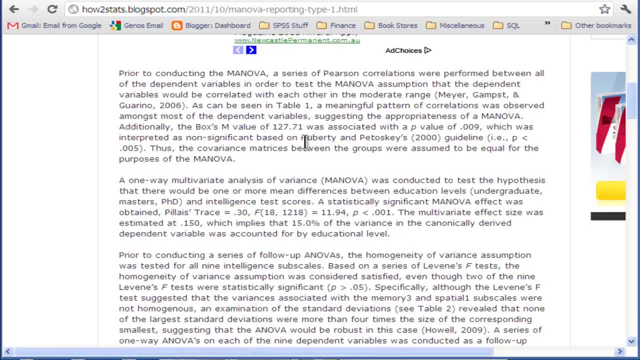 and that's to test the hypothesis that the covariances are the same amongst all groups, that is, the covariances amongst the dependent variables. But I've got a reference here in the results section from Huberty and Petowski saying that the boxes M value you wouldn't evaluate at an alpha of .05, but instead at .005.. 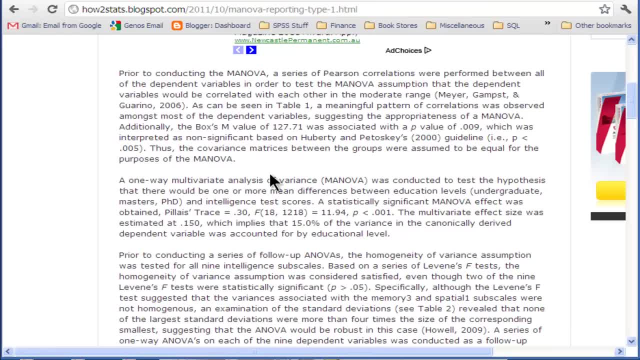 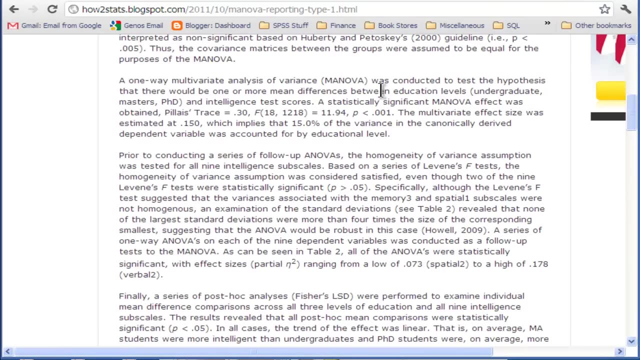 So it's tougher to reject the null hypothesis. And in this case we don't actually want to reject the null hypothesis. We want the assumption of homogeneity of covariance matrices to be true. So I've got a little book, little section on that with a useful reference. Then I go into the MANOVA and I report the results. 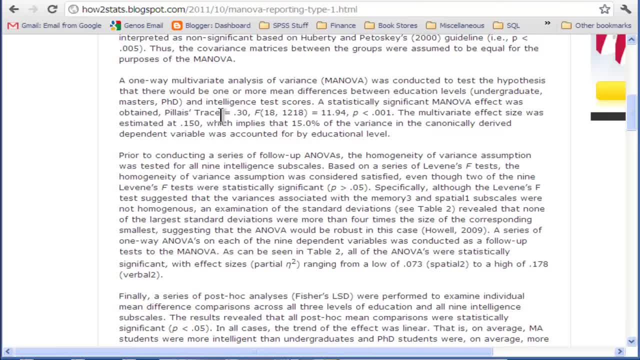 and I reference: you make use of place trace, which is the most robust of violations of the covariance matrix assumption, But my sample size was so huge I felt confident of using it. I suspect in other cases people will be tempted to use Wilkes-Lambda, which is totally fine. You probably 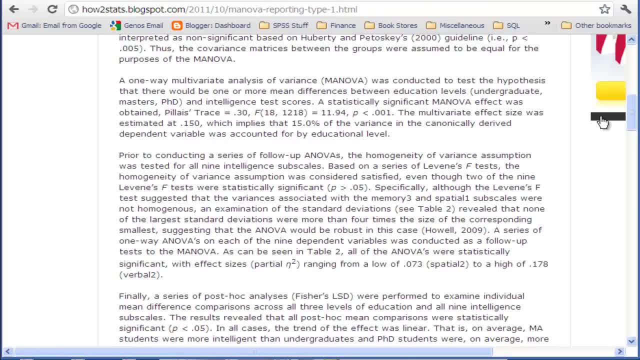 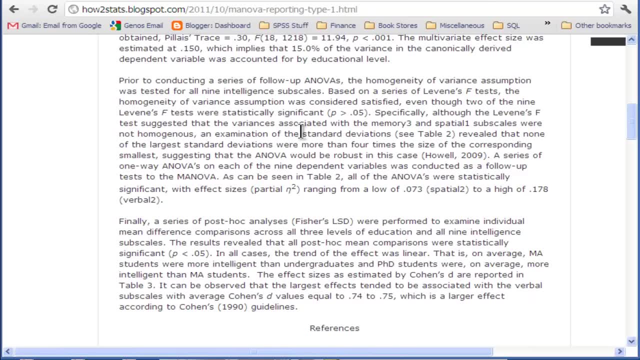 see that just as often as you do place trace, Then because this is not the interesting sophisticated way of doing a MANOVA, it's just doing a MANOVA to help protect against the chance of making a type 1 error In the video. I say if you've convinced yourself and others that that's the 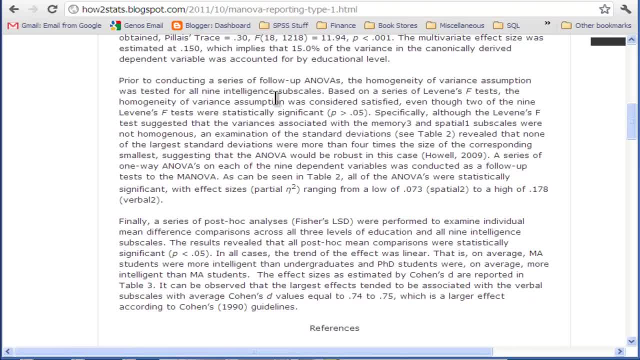 way to do it, then here's how you'd report it. So here I've got the ANOVAs, but before I do that, I'm going to show you how to do it. I'm going to show you how to do it. I'm going to. 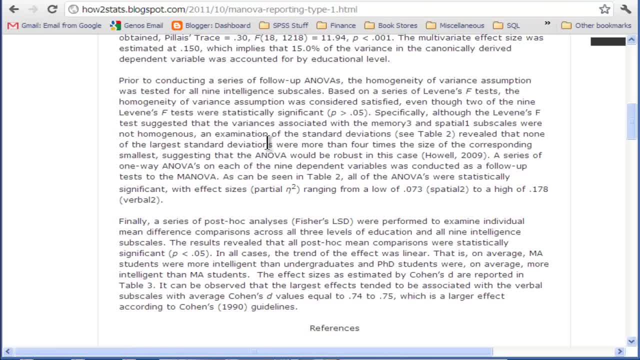 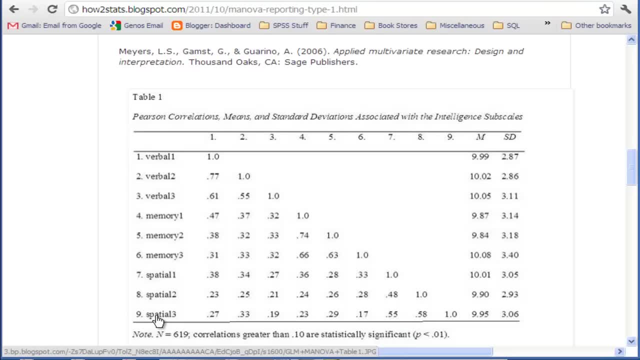 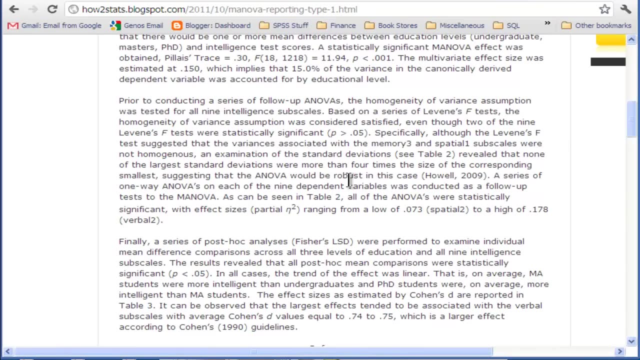 do that. I actually report Levine's F test because I have to test the assumption of homogeneity, of variance, for the nine ANOVAs that are now going to be performed on all these nine dependent variables across the three levels of education And I find that none of them, I think I found 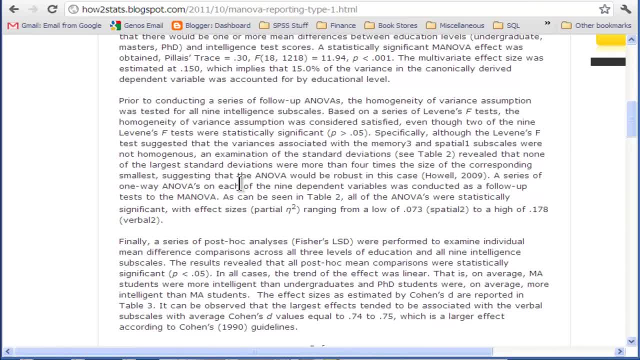 two of them rejected the null hypothesis of homogeneity of variance. But then I cite Howell, 2009, who, based on his summary of the research, says that if you don't have one standard deviation or variance four times larger than the smallest, then you should feel confident of doing the ANOVA and that the p-value associated with the ANOVA will. 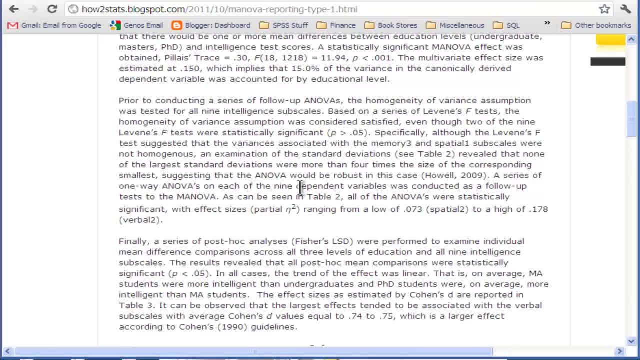 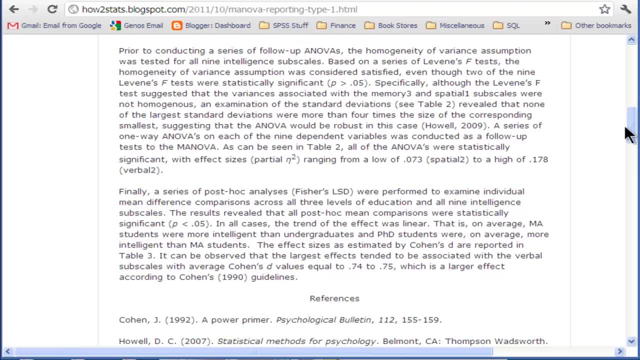 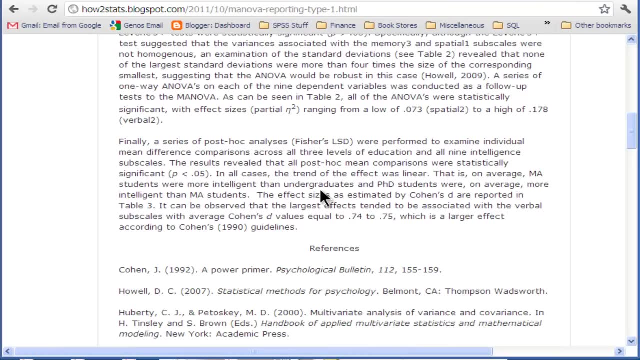 be relatively accurate. So that's a key statement here, that the homogeneity of assumption was violated, but the standard deviations were still not four times greater. So I've got Howell 2009 for that. And then, finally, you're doing a series of post-hoc analyses and I 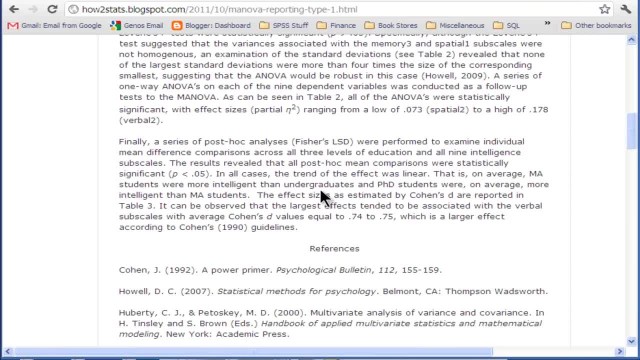 chose Fisher's LLT Because if you've convinced yourself that the ANOVA protects you against making type one errors, if it's statistically significant, then why not go for the most powerful statistic? Some people might say: well, you should use two keys, or maybe some kind of hybrid Bonferroni.